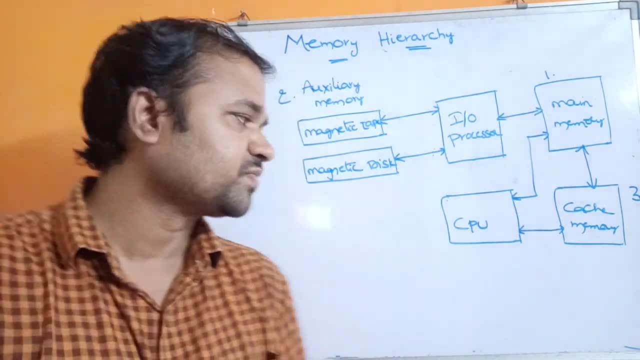 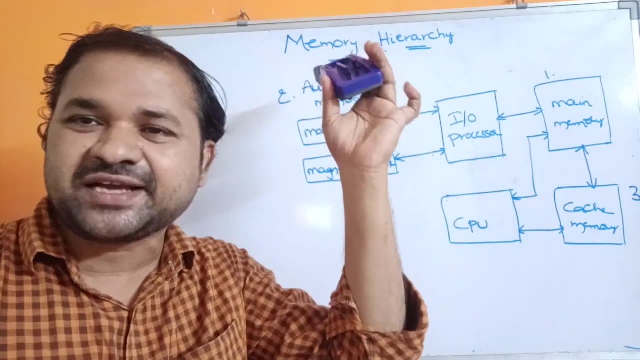 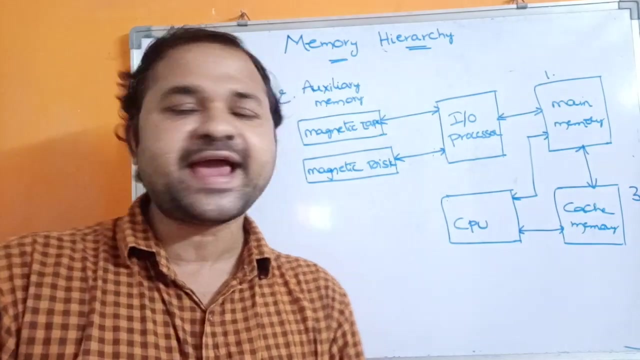 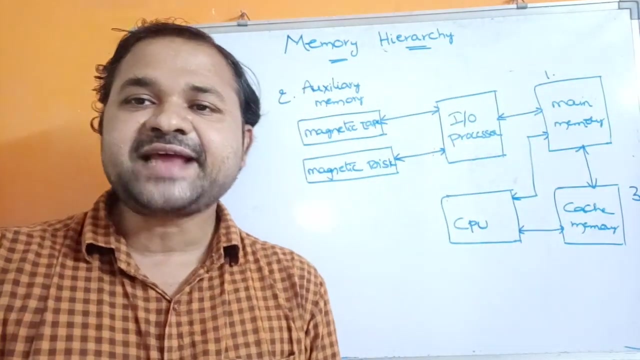 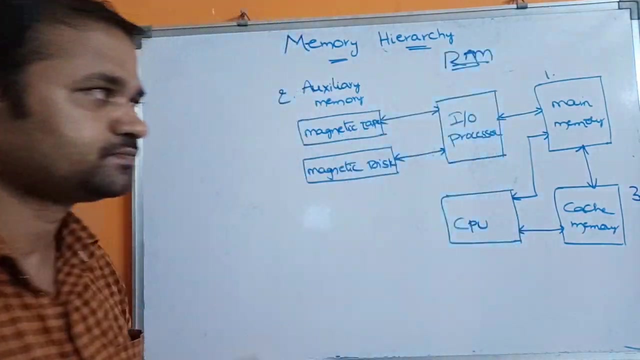 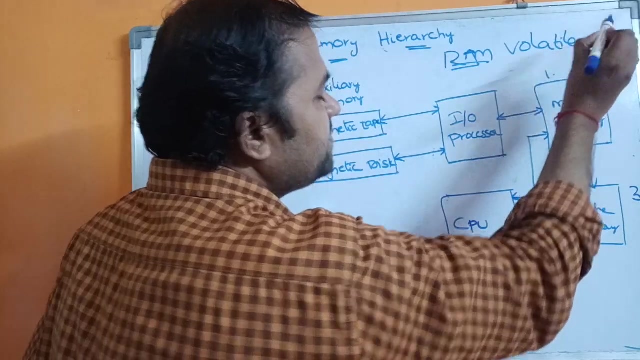 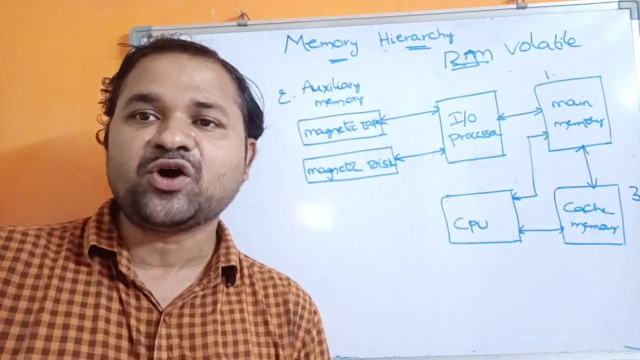 But CPU can execute a program only if the program presents in main memory only. Suppose if the program present in auxiliary memory or secondary memory, then CPU cannot access the data. So CPU can access An instruction If that instruction is present in main memory only. The best example for the main memory is RAM. RAM stands for random access memory. Main memory is called as volatile memory. Main memory is called as volatile memory. So that means whenever we switch off the computer then the entire content of the main memory will be lost. 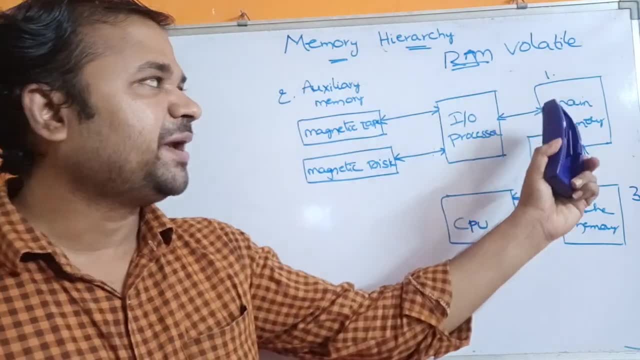 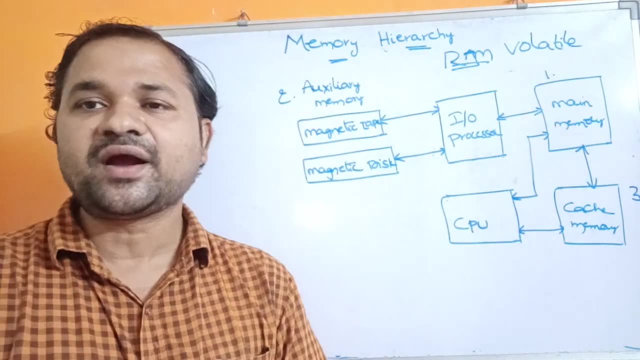 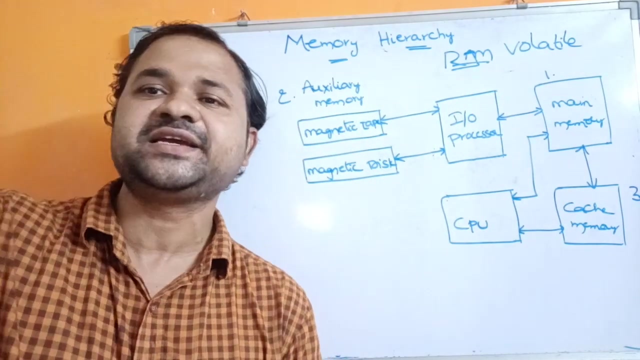 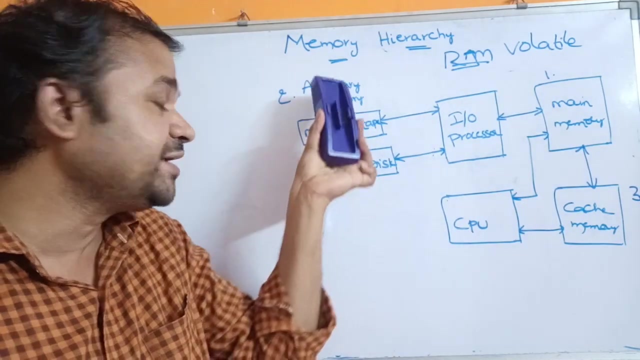 So that is about main memory. Main memory can also be called as primary memory, also Because main memory is really very important in order to execute the instruction by the CPU. 17, 00 as a. If you take any program, either CE or C++ or Java, or it may be any program, whenever we save the program, then the program will be stored. it secondary. 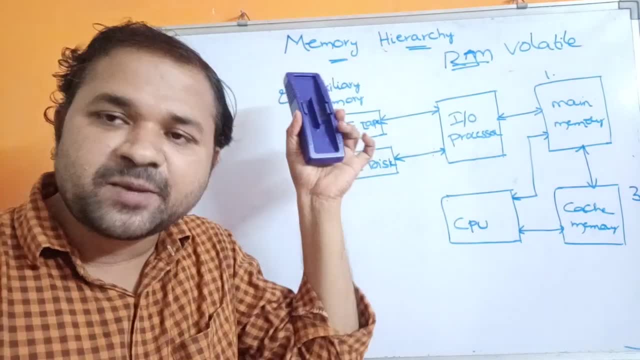 memory During compilation also. the program will be saved in important secondary memory. during compilation also. the program will be saved in important secondary memory because it has mingled with other chip, So that means I will read it as primary memory. Uh, that is about main memory. 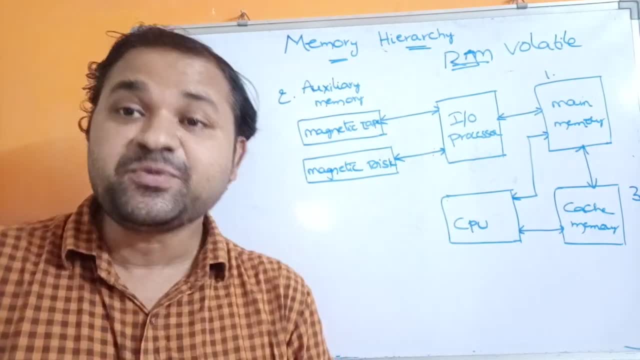 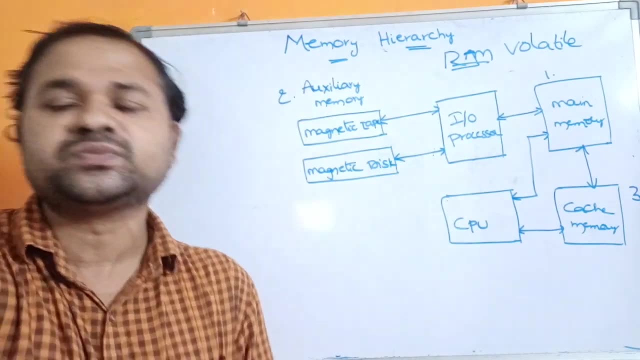 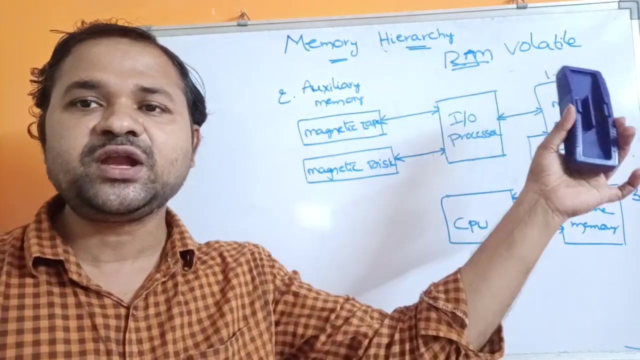 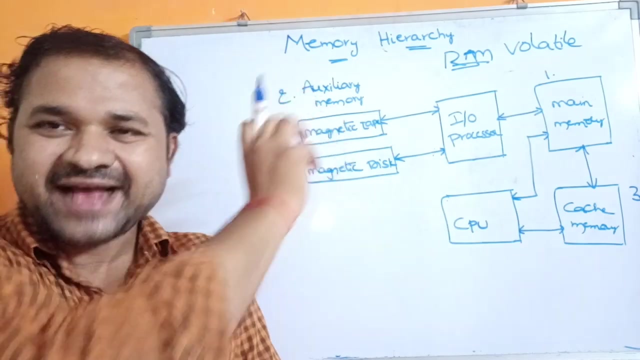 in secondary memory only, but at the time of execution, operating system or DMA, transfers that program from hard disk to main memory. why? because CPU has to execute the program. CPU executes the program only when the program resides in main memory only now let's talk about axillary memory here. this axillary 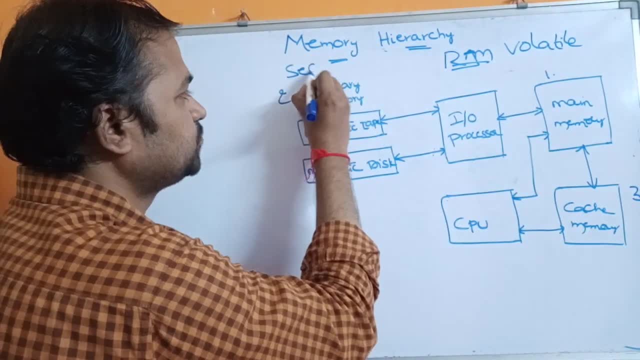 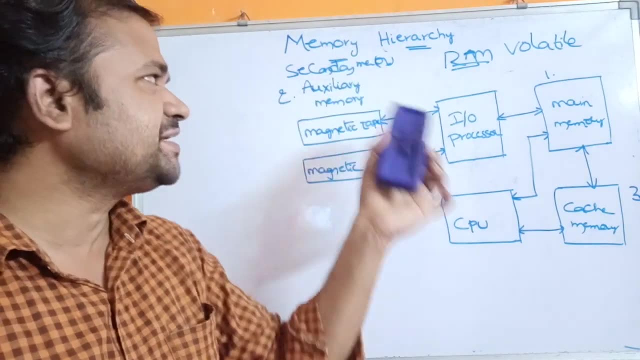 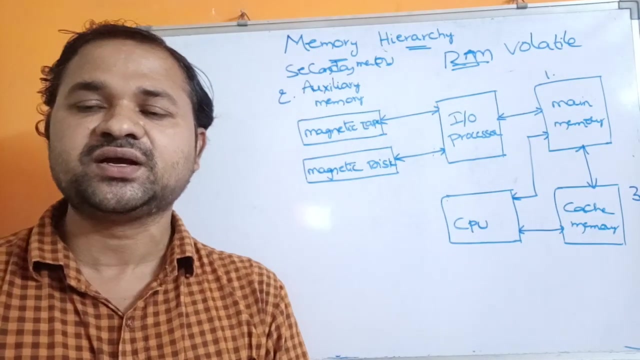 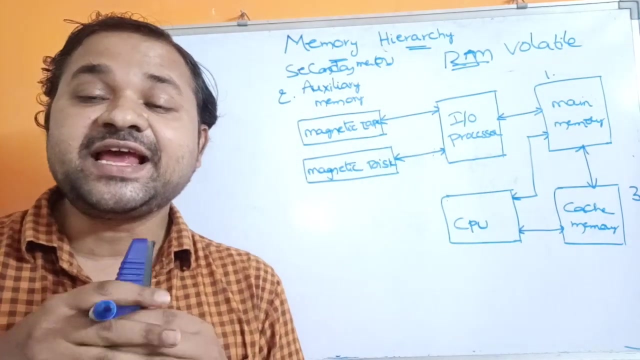 memory can also be called as secondary memory also. this axillary memory can also be called as secondary memory also. let's see what is the advantage of the axillary memory. auxiliary memory or secondary memory is mainly useful in order to store the data permanently in the computer. so that means axillary or. 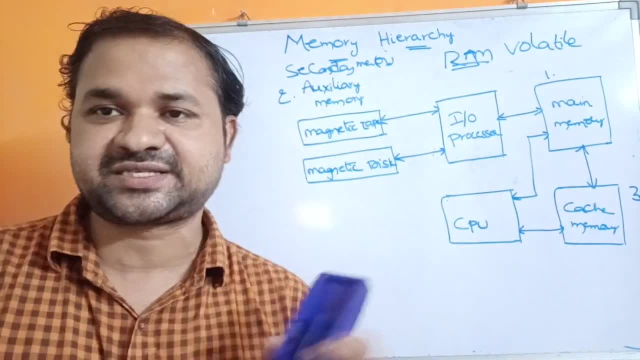 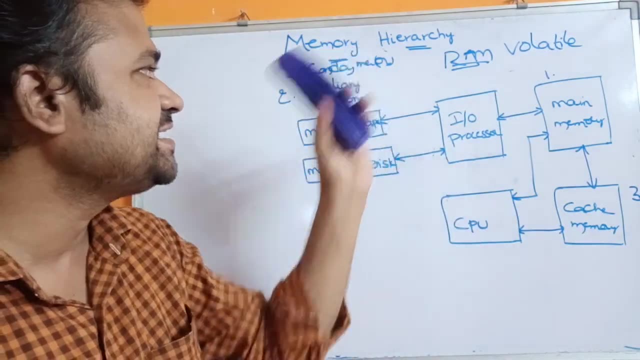 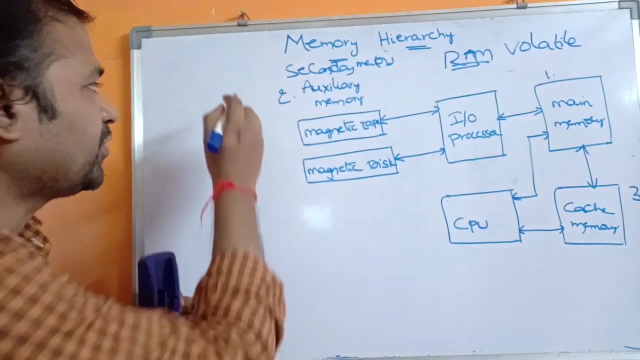 secondary memory is useful for backup purpose. so in order to store the data permanently in the computer, we use this axillary or secondary memory. axillary memory can also be called as non volatile memory. why? because when we switch off the computer, then the content of the axillary or 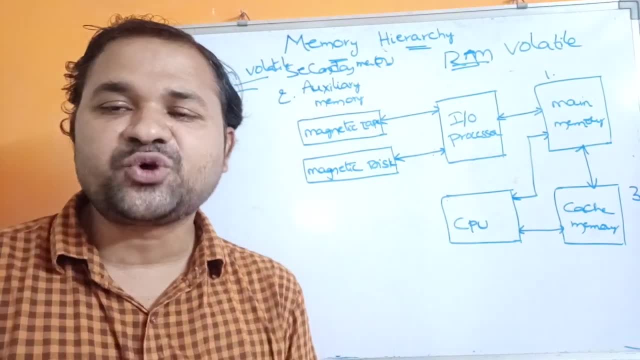 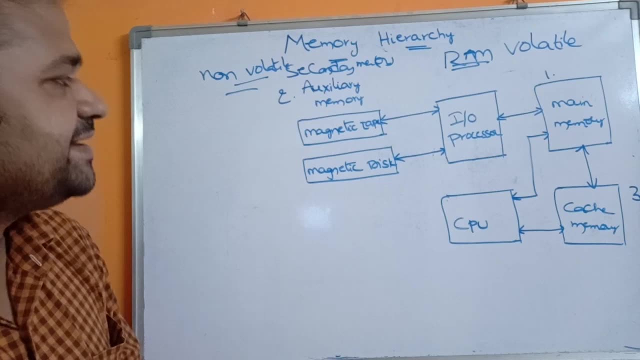 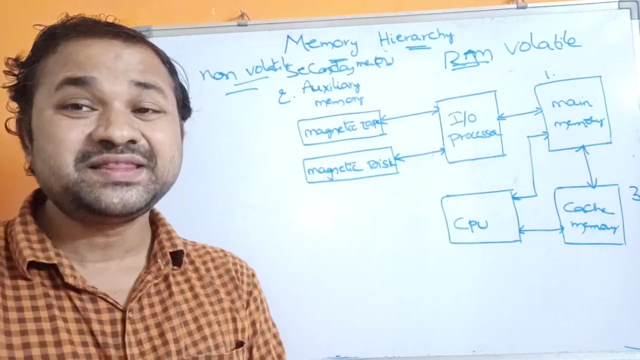 secondary memory will not be lost. they will be stored permanently in the computer, unless we deleted the data. and the best examples for the axillary or secondary memory are magnetic tape, magnetic disk. magnetic disk is nothing but hard disk. in the older days we use a magnetic tape, but nowadays we are using magnetic disk only. 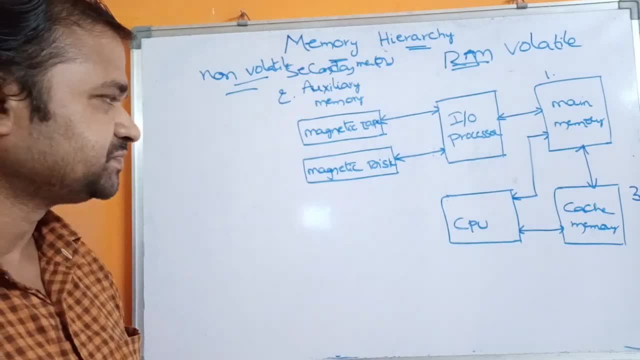 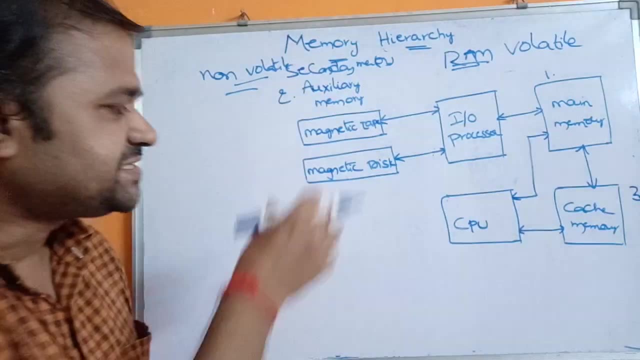 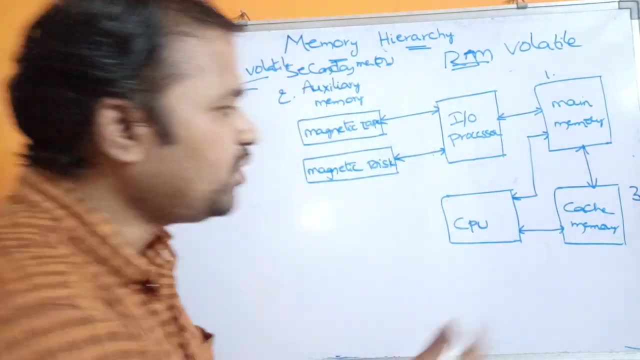 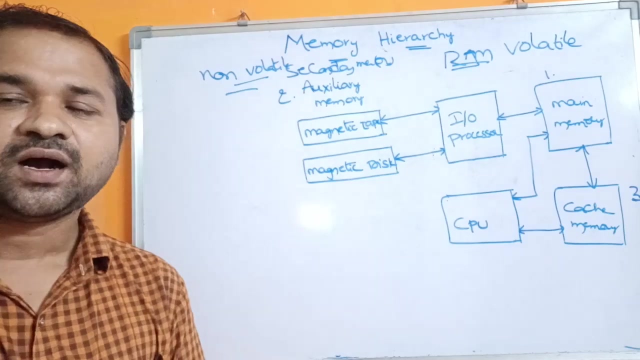 so magnetic disk is nothing but hard disk. so this is useful in order to store the data permanently in the computer, but CPU cannot access the data. CPU cannot access the data which is present in secondary memory. now let's see about cache memory. cache memory is a small and faster memory. 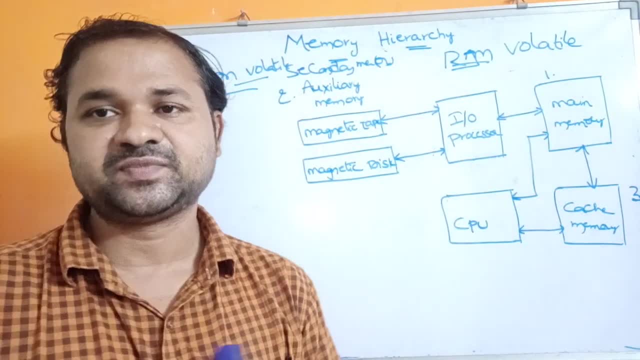 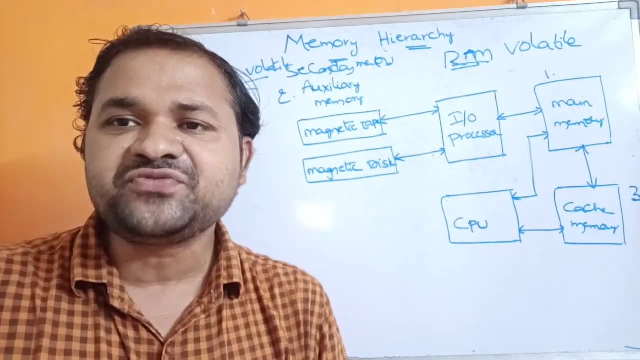 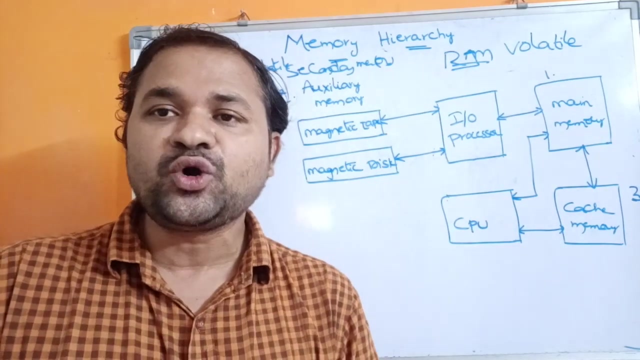 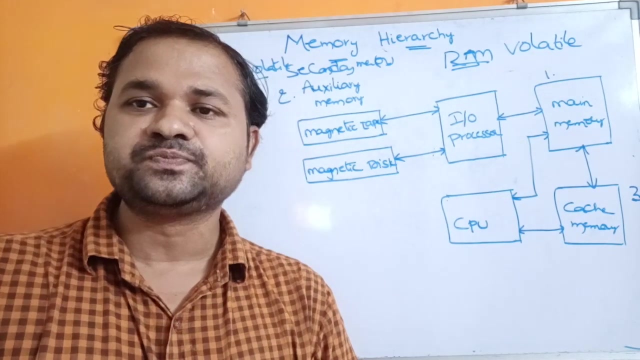 which has higher accessibility. here. the cache memory is very, very faster memory, but the size of the cache memory is very, very small. cache memory is mainly useful in order to store frequently used instructions. let we use a, c for loop, for i is equal to 0, i less than 100, i plus plus. so how many times we are? 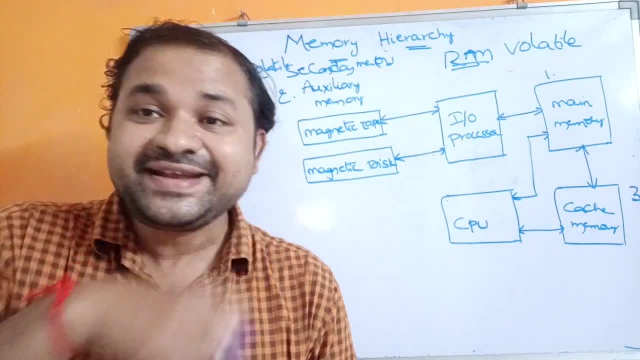 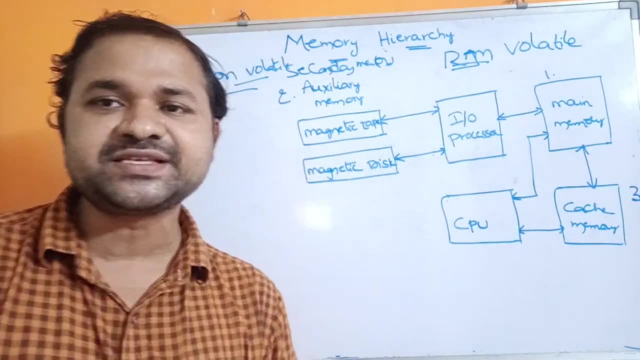 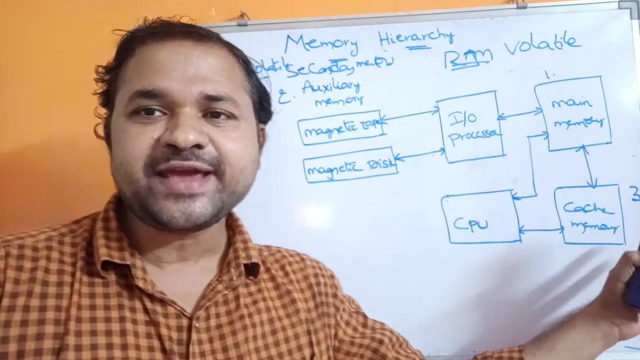 repeating that for loop 100 times. so 100 times we have to use the value of i. so in that occasion what the operating system will do is: operating system transfers that instruction into the cache memory. here the cache memory access time is extremely faster, so cpu can access the data of. 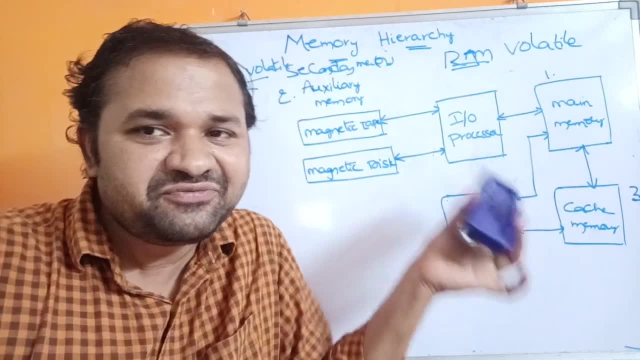 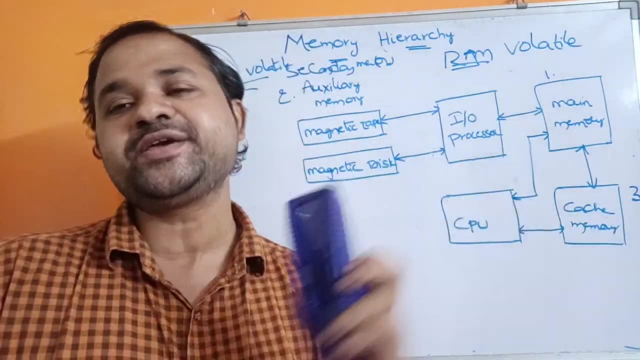 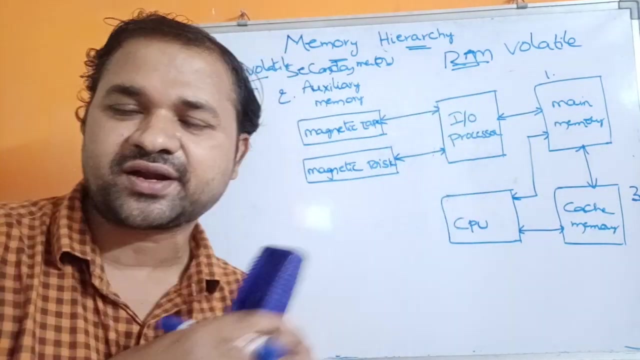 the cache memory in a faster manner than if the data presents in main memory. main memory access time is slower when compared with cache memory access time. so if there are any frequently used instructions, then operating system or i o processor or direct memory access dma transfers those instructions to the cpu and then the cpu can access the data of the cache memory. 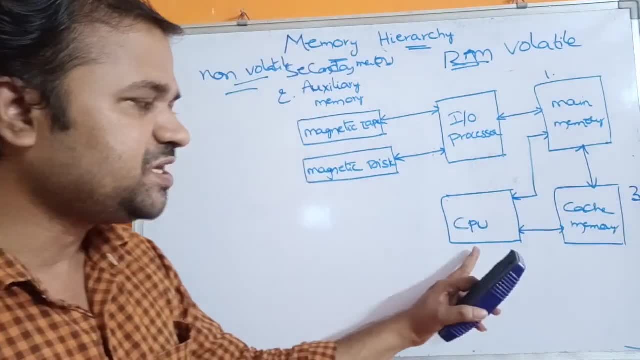 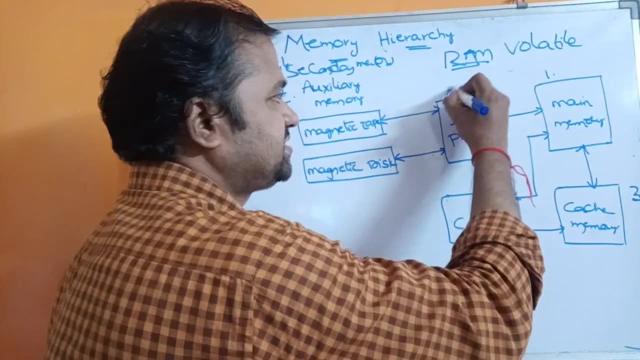 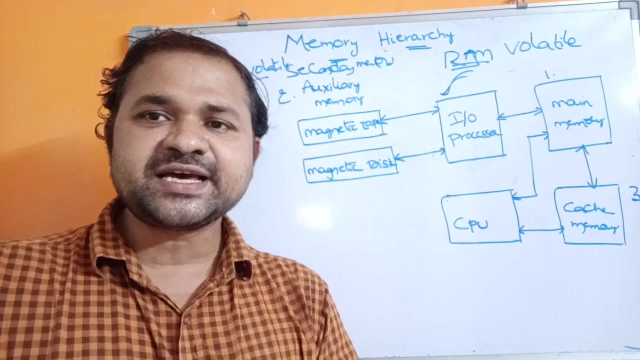 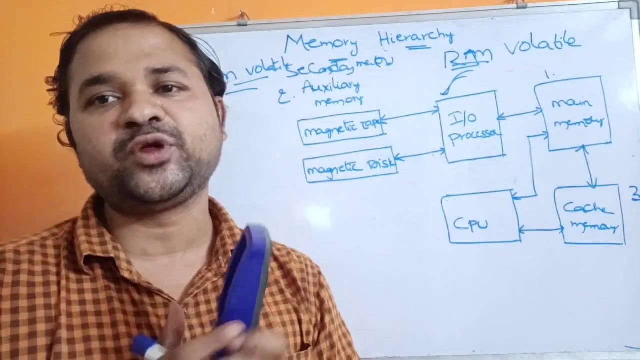 instructions from main memory to the cache memory so cpu can access that instructions in a faster manner. now let's take the let's. let's now, let's take. what is the use of i o processor- input output processor. i o processor is mainly useful in order to transfer the data from hard disk to main memory. 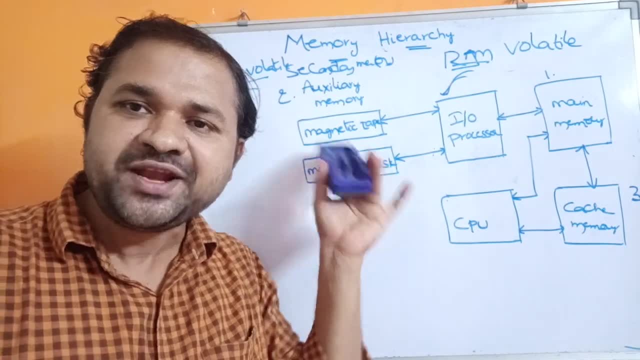 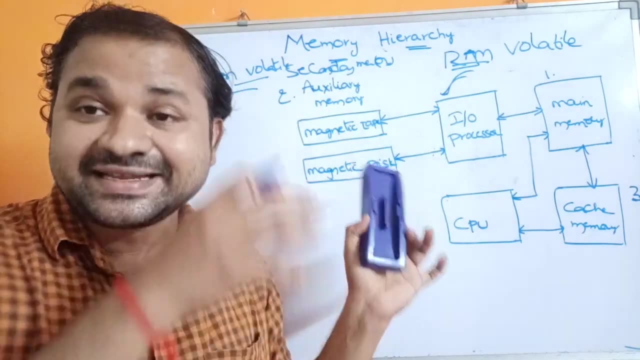 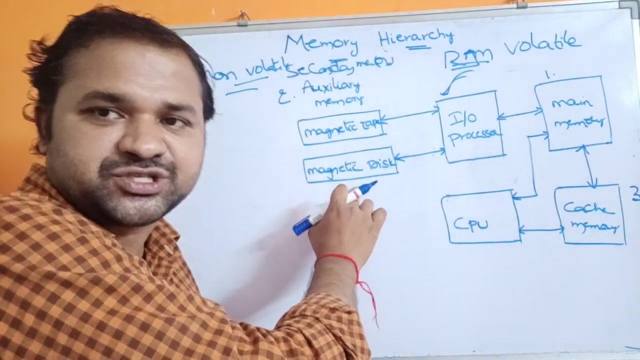 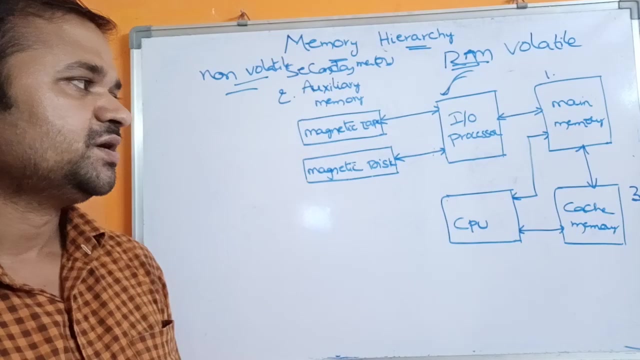 whenever we save the program, then the program will be stored in hard disk only during compilation also the program will resides in hard disk. but at the time of execution i? o processor will transfers the program which is in hard disk to main memory so that cpu can execute the program which is present in main memory. so i? o processor is mainly useful in 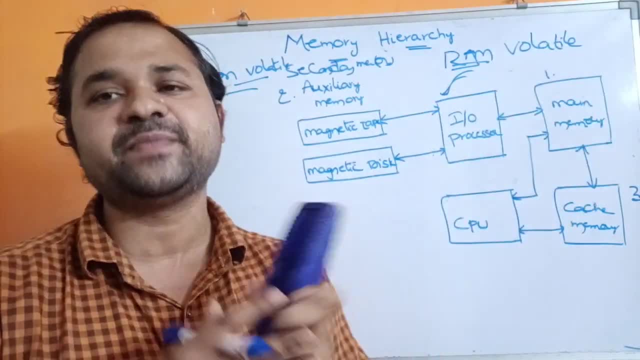 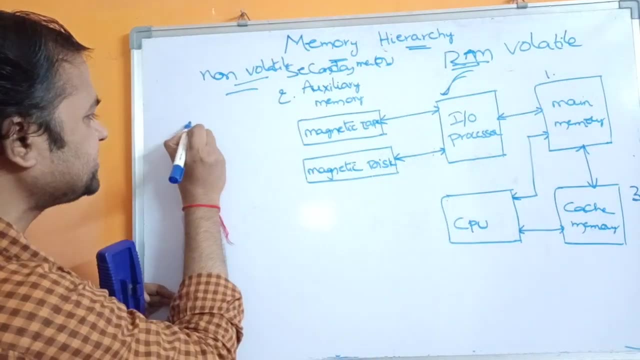 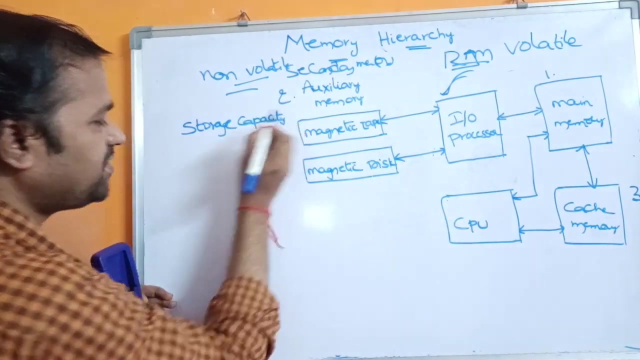 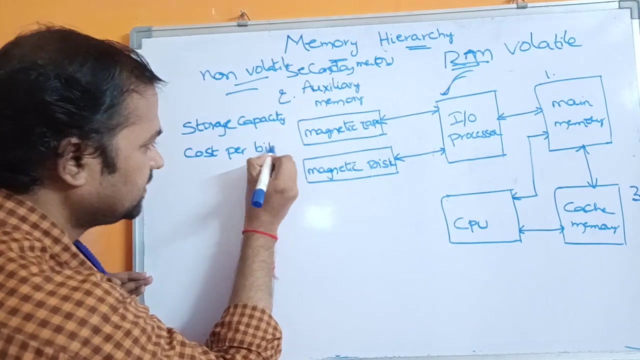 order to transfer the data from secondary memory to the main memory. now let's talk about the properties of the i o processor in order to transfer the data from secondary memory to the main memory. just talk about the properties of this memories mainly. we will discuss three properties here. the first property is: 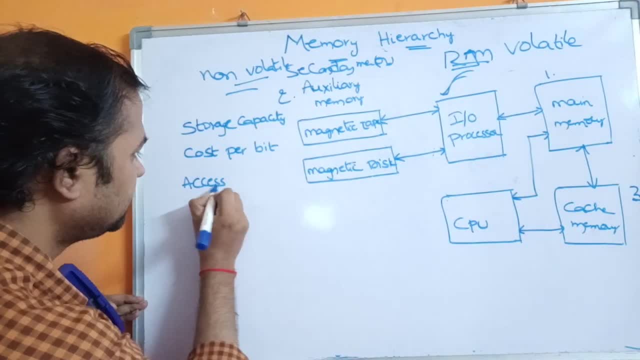 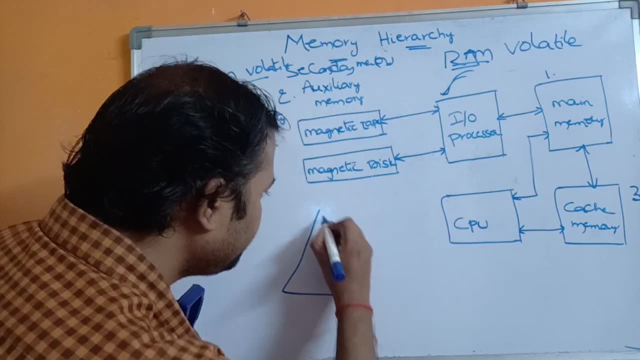 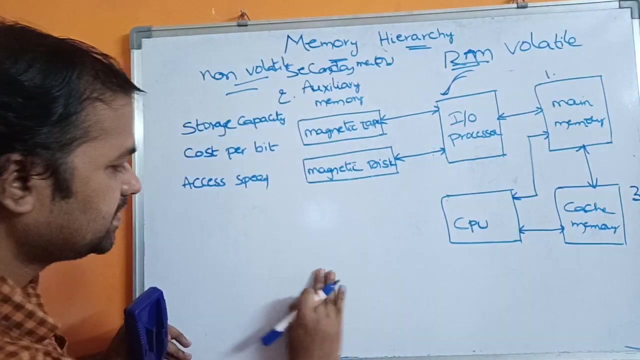 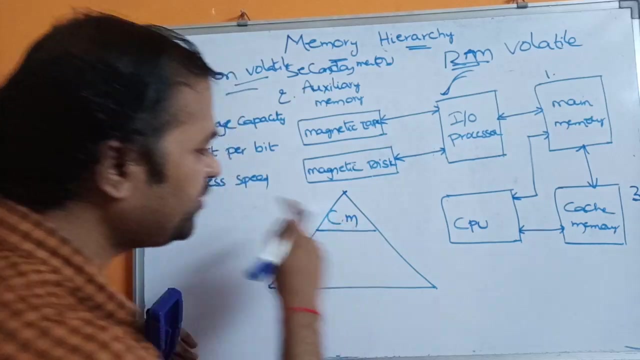 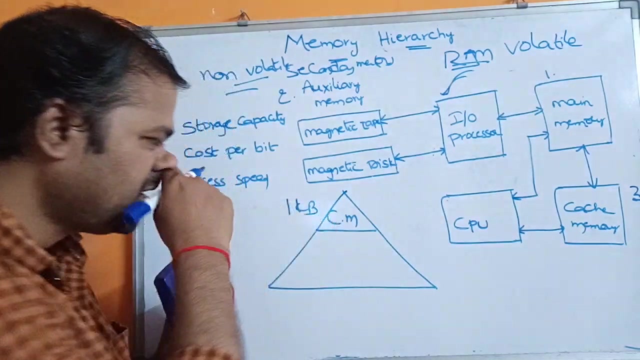 so the next property is easily the access speed those memories. i'm using a diamond symbol like this: here the first memory is cache memory, so the first memory is catch memory. here the catch memory storage capacity will be in the kb's, like 128 kb, 256 kb. 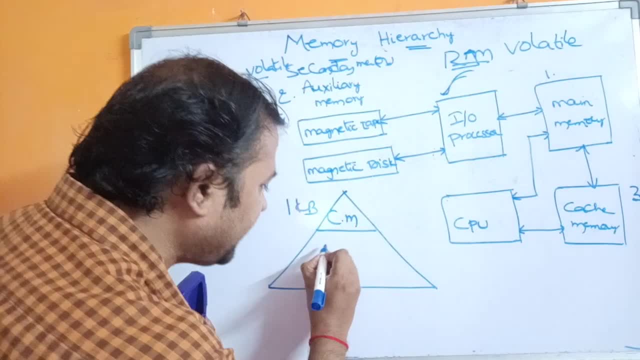 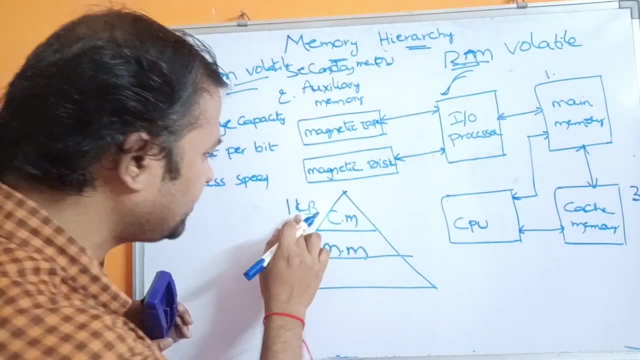 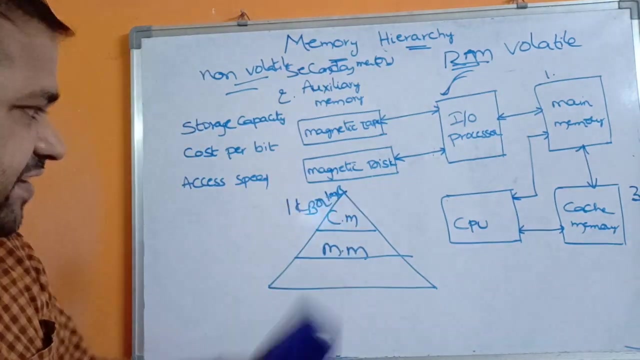 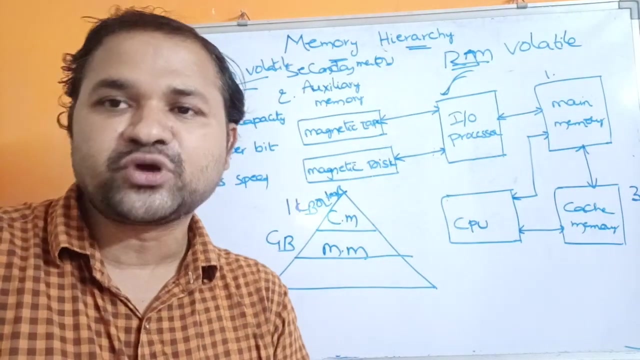 512 kb, like that, and the next memory is main memory. main memory storage capacity will be in here. the cache memory storage capacity is in kb's or we can also use like 1 mb, 2 mb, like that also, whereas the main memory storage capacity will be in gb's, like 2 gb, 4 gb, 6 gb, 8 gb, 16 gb, up to 32 gb. 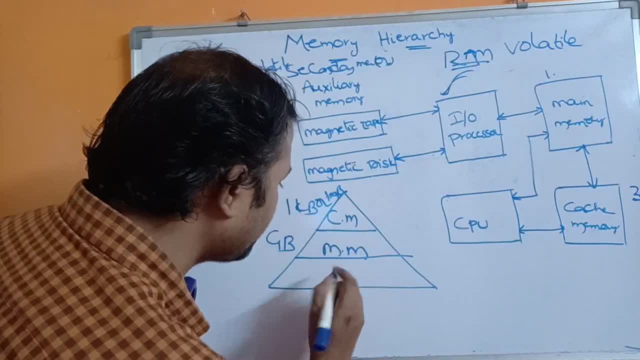 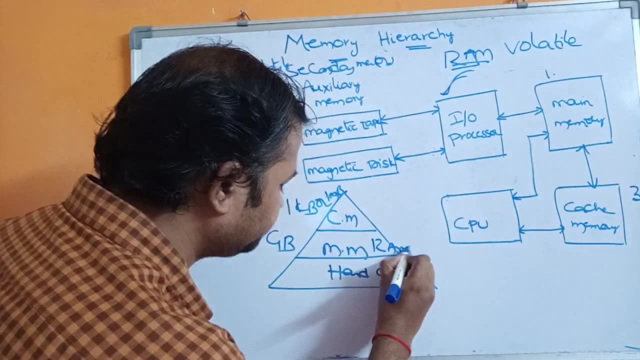 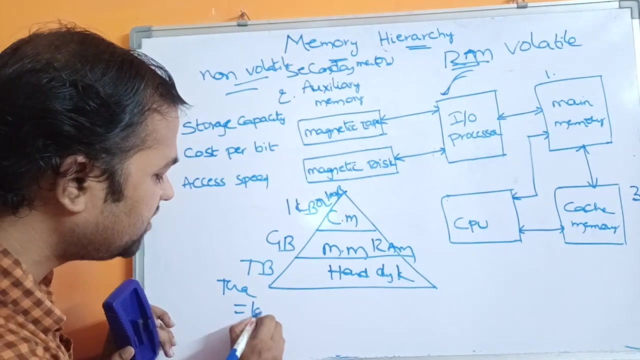 also we can use. and the next one is secondary memory. that is nothing but hard disk. secondary memory, that is nothing but hard disk. main memory is nothing but ram. the hard disk capacity will be in pbs. tv stands for terabyte, so one terabyte is equal to 1024. 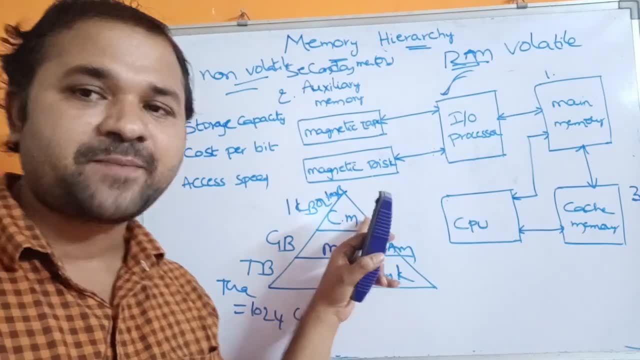 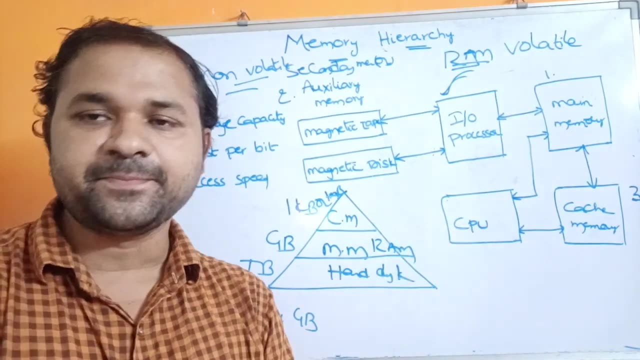 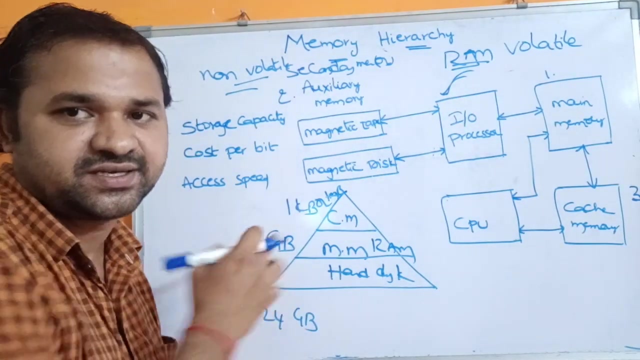 gigabytes, so here the. the storage capacity of the cache memory will be in kb's as well as mb's, kb's as well as mb's, so 1 mb is equal to 1024 kb. various main memory capacity will be in gb's, so 2 gb, 4 gb 8, gb 16 gb 32. 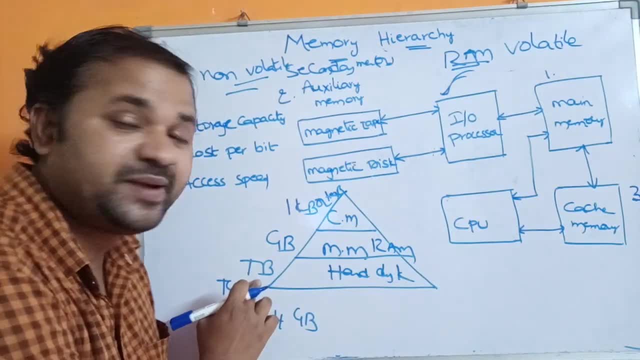 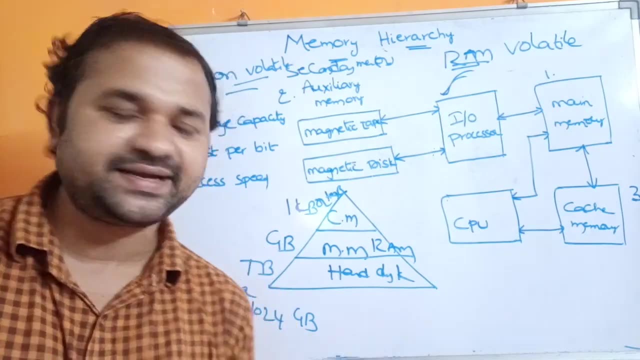 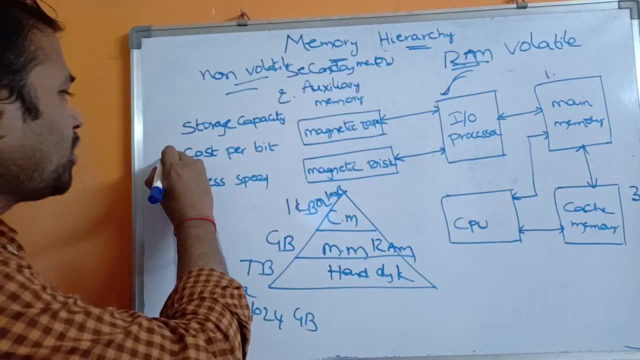 gb. like that. hard disk storage capacity will be in terabytes, so 1025 gigabytes, 500 gigabytes, 300 gigabytes, like that. the hardest storage capacity will be like that. so this is about the storage capacity. now let's see about the cost here. 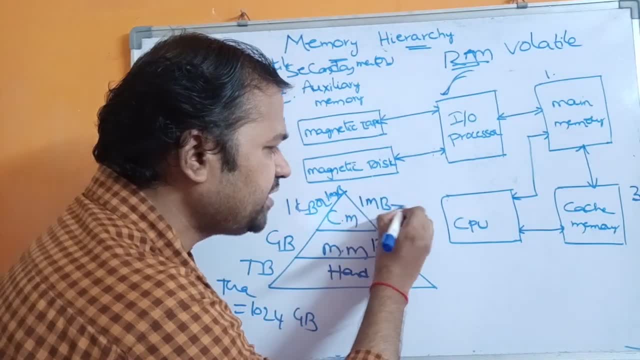 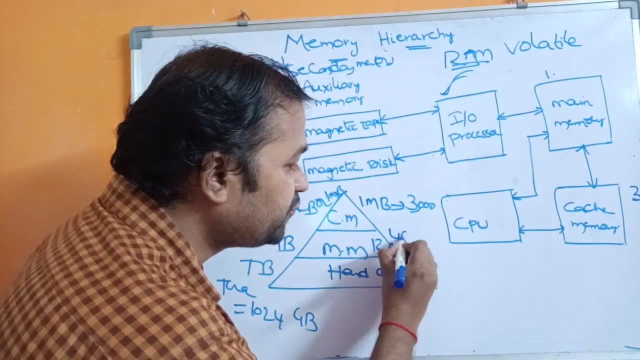 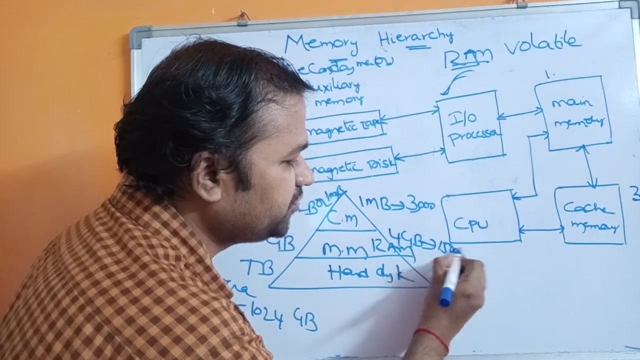 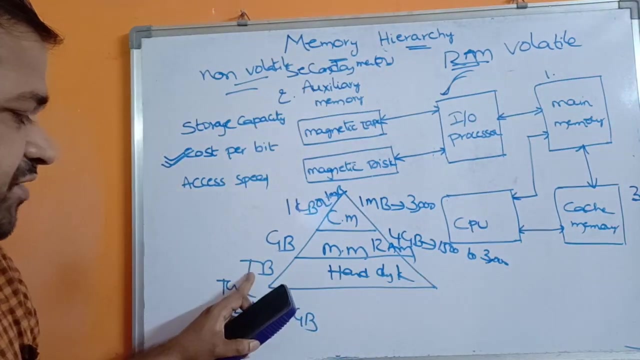 here, in order to buy 1 mb of the cache memory, we need to pay some 3000 rupees, whereas in order to buy 4 gb of the main memory- with the help of some- some 1500 to 1500 to 3000- we can buy 4 gb of the ram, whereas in order to buy 1 terabyte of the hard disk or external. 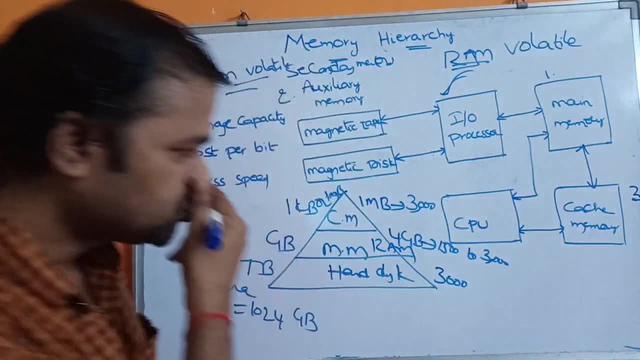 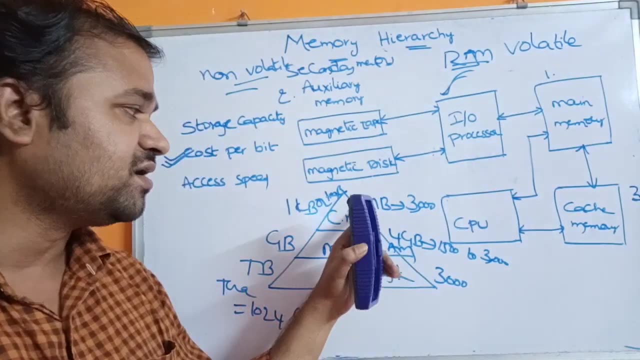 memory. we can use some 3000 rupees memory here. in order to buy 1 mb of the cache memory, we need to pay 3000 rupees. so here the point is: cache memory is very, very expensive. in order to buy 1 mb of the 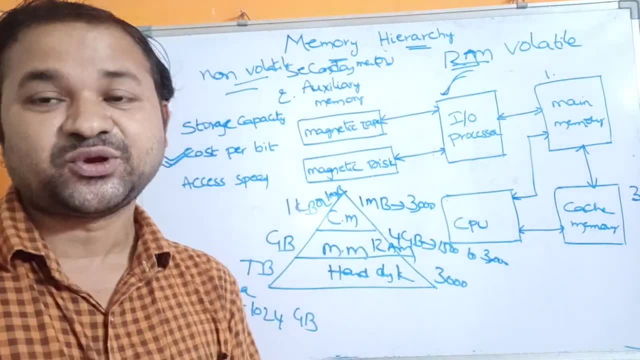 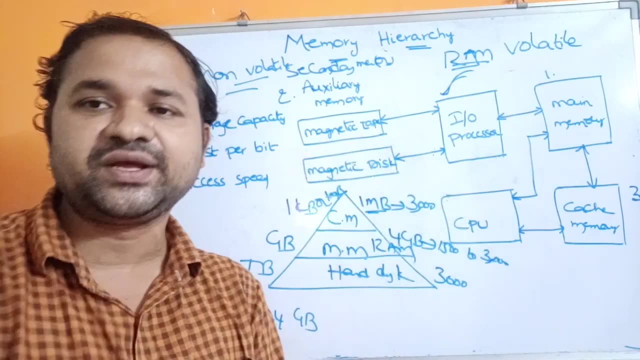 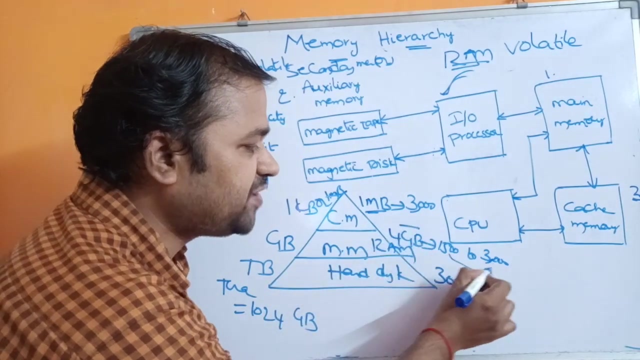 cache memory, we need to pay 3000 rupees, so it is very, very expensive. in order to buy for 1 mb only, it stores only 1 and b a data only, whereas this ram, for 4 gb of the ram, we have to pay from 1500 to. 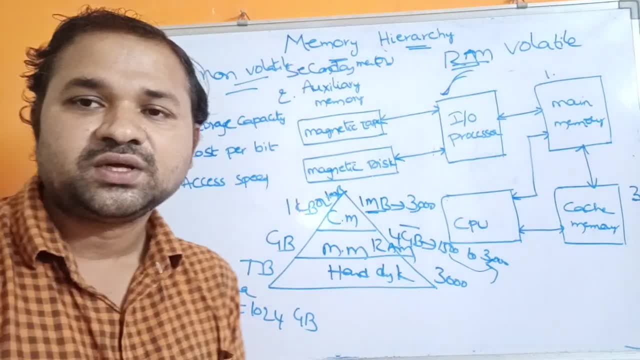 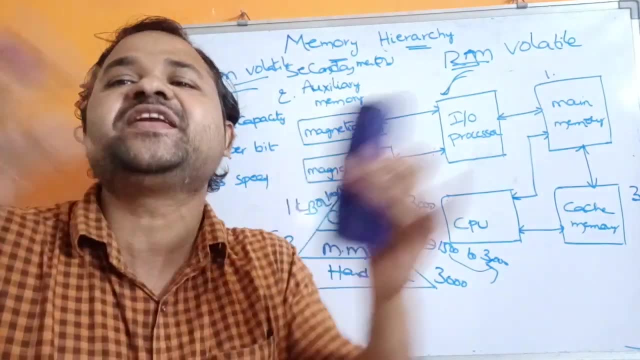 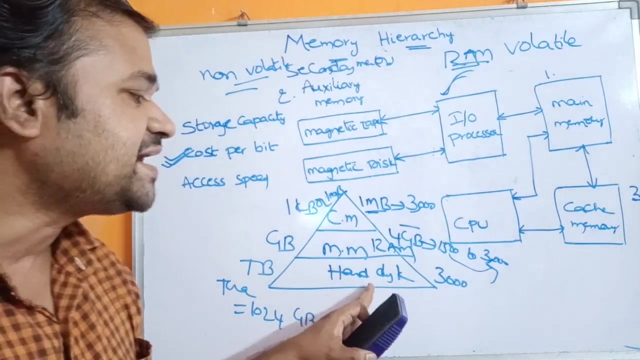 1500 rupees. so that means main memory is also relatively expensive when compared with this one cache memory. cache memory is very, very expensive, whereas main memory is little bit less expensive when compared with this main memory, whereas hard disk- hard disk- is very, very cheaper in order to 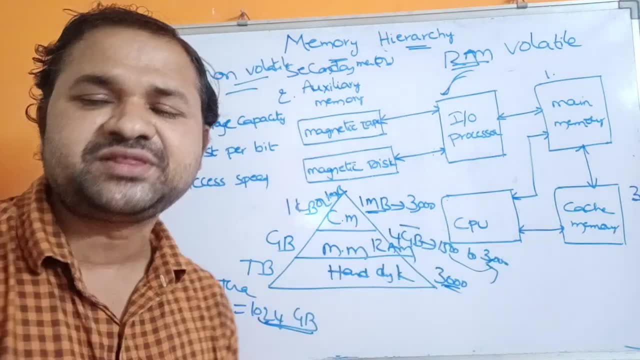 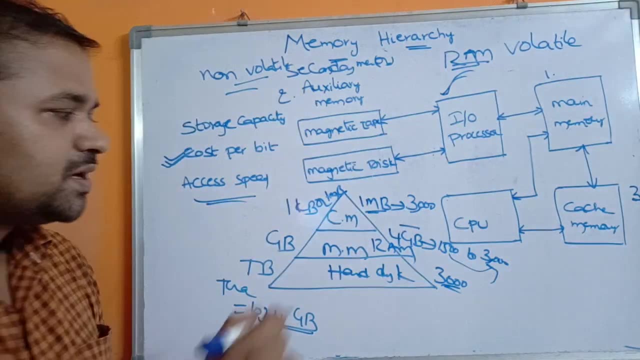 buy 1024 gb of the artist, you need to pay only 3000 rupees only. okay, so this is about the cost of each and every device. now let's see about the cost of each and every device. now let's see about the access speed. here the cache memory is extremely faster, but the problem with the 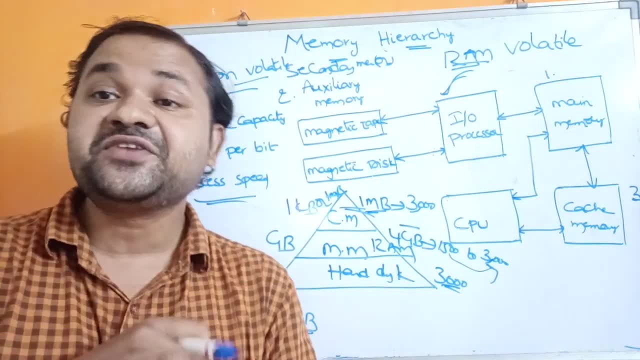 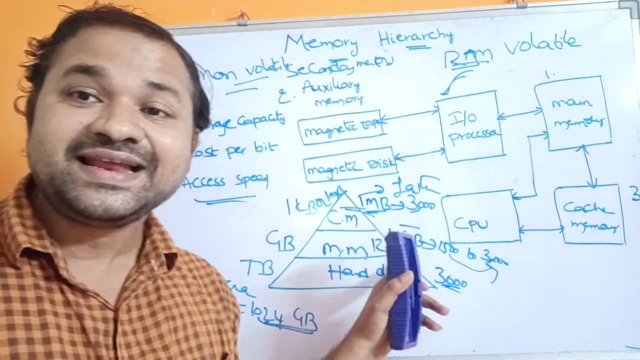 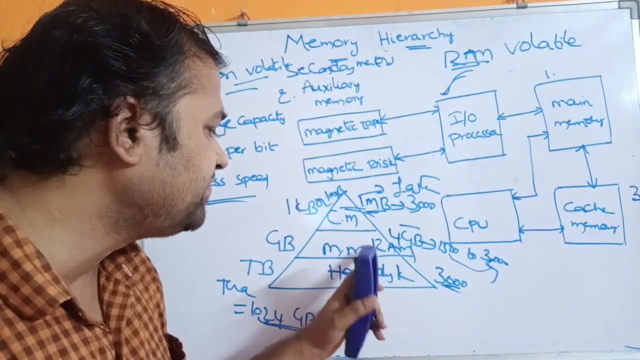 cache memory is: it is very, very expensive. it is very, very expensive. so this cache memory is very, very faster. main memory is relatively slower than the cache memory. hard disk is very, very slower when compared with main memory. so here cache memory is very, very faster. main memory. 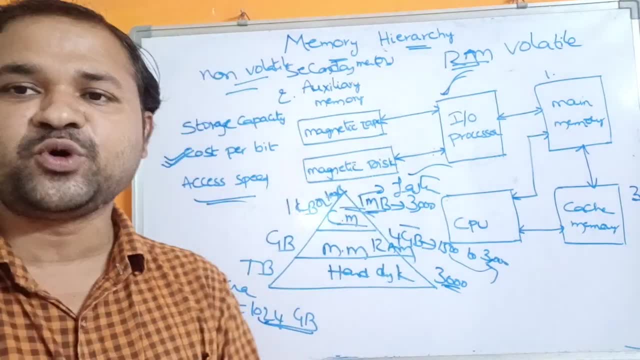 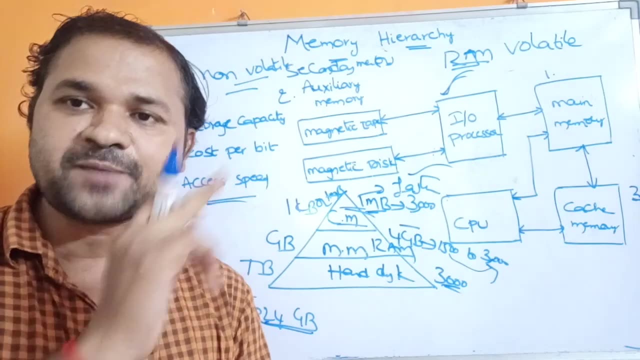 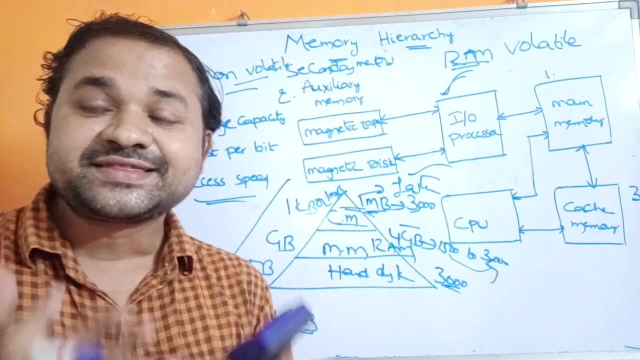 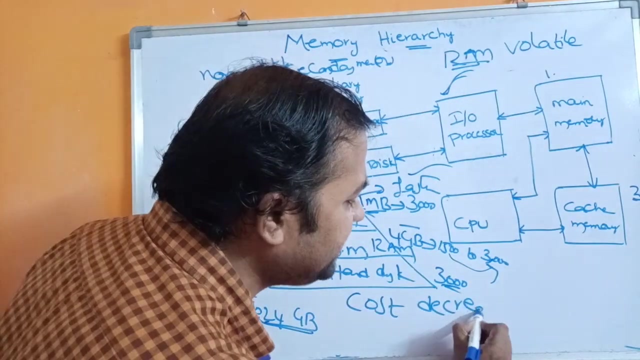 is relatively slower than cache memory. hard disk is very, very slower when compared with main memory and the cache memory. so here the point is: yes, the storage capacity of the memory increases. yes, the storage capacity of the memory increases, the cost will decrease. the cost will decreases as well as. 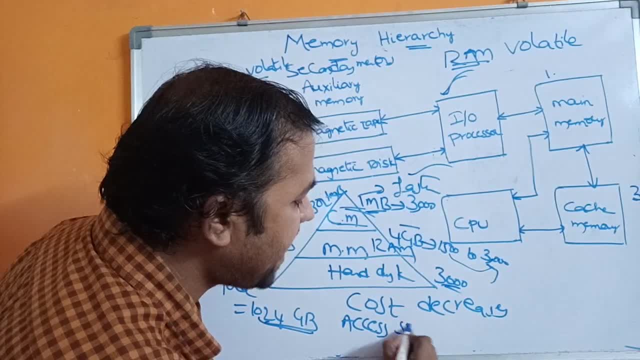 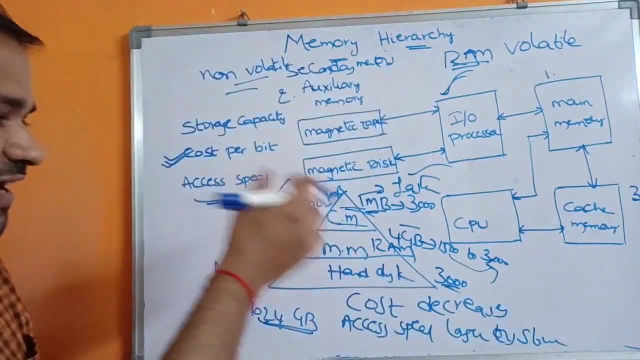 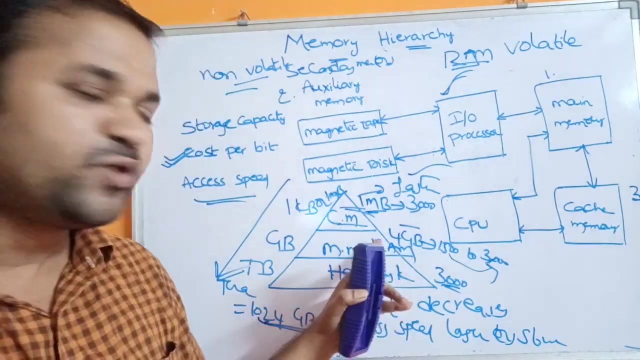 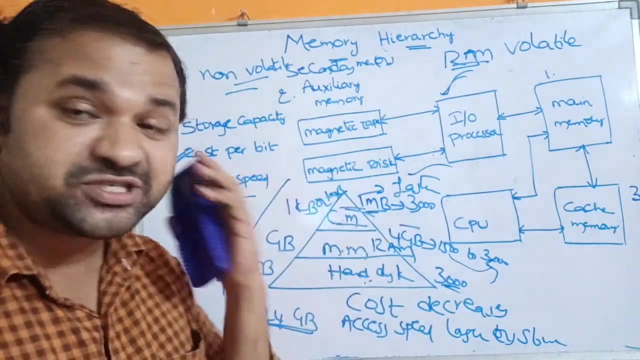 access speed also becomes slower. access speed also becomes slower or longer, so longer or slower. so here, if you take hard disk, hard disk storage capacity is very, very, very, very high. main memory storage capacity is somewhat high, when somewhat high when compared with the cache memory. cache memory storage. 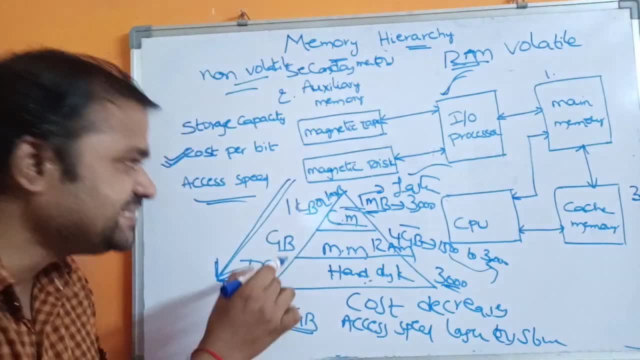 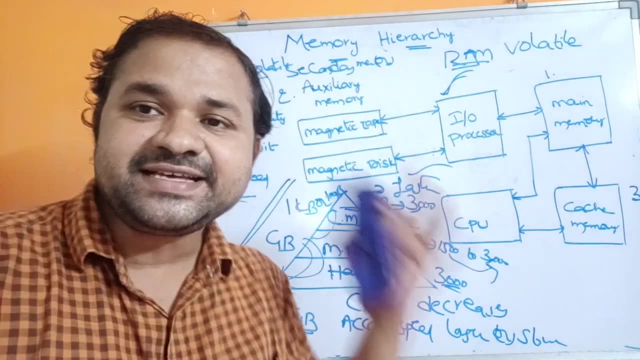 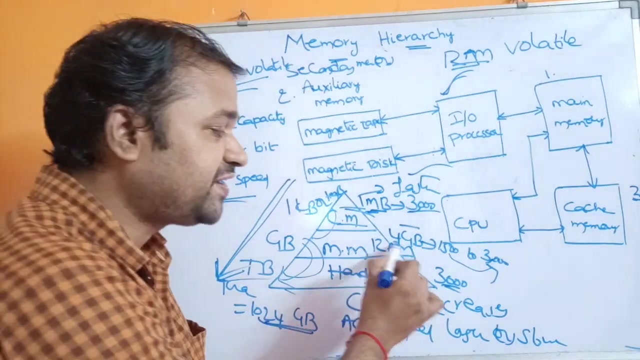 capacity is very, very low. so here, as the storage capacity is increasing, from mb to gb, from zero, from gigabyte to terabyte, then the cost is decreasing. the cost is decreasing. so here for m for one mb, we are using 3000. here for 4gb, we are using 3000. here for 1024 gb, we are using 3000, so the cost is. 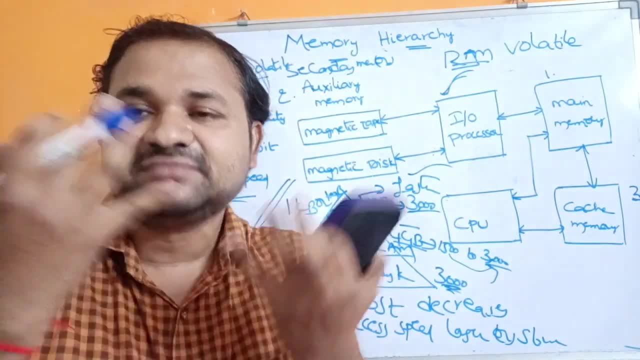 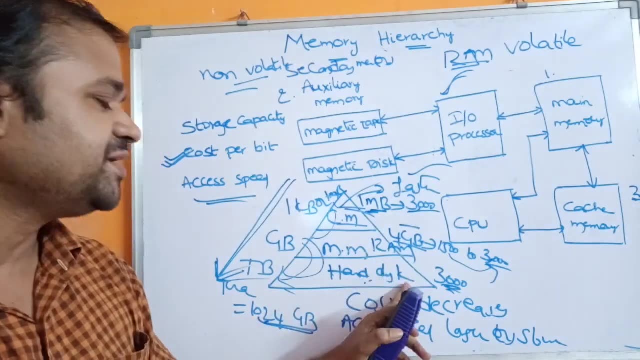 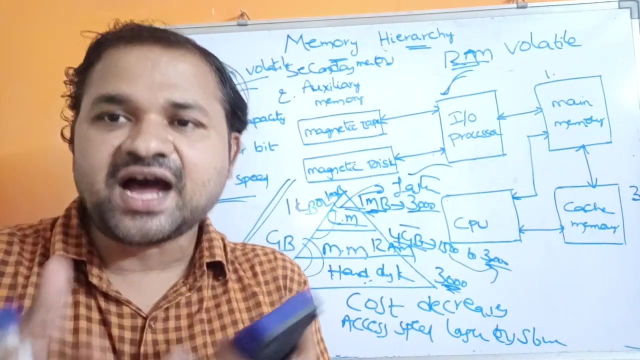 decreasing as well as access speed is also becoming decreasing. so here the access speed is extremely faster. it is slower when compared with this one. it is extremely slower when compared with these two memories. so why we are using all these memories is: with less cost we need to produce average. 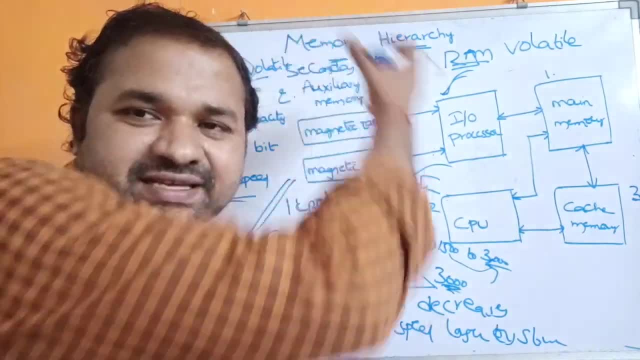 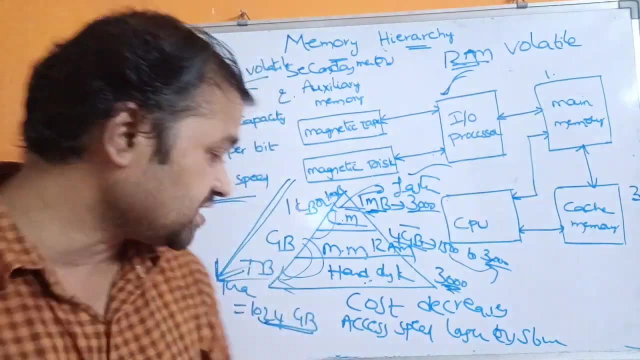 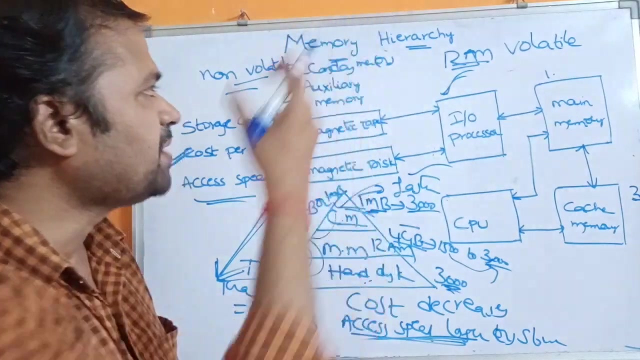 performance. so why we are using this, these many types of memories. so this is the main point here. so, with less cost, uh, we need with less cost as well, as we need to produce for some average performance, uh, and here we are using memory hierarchy mainly to implement multi programming. 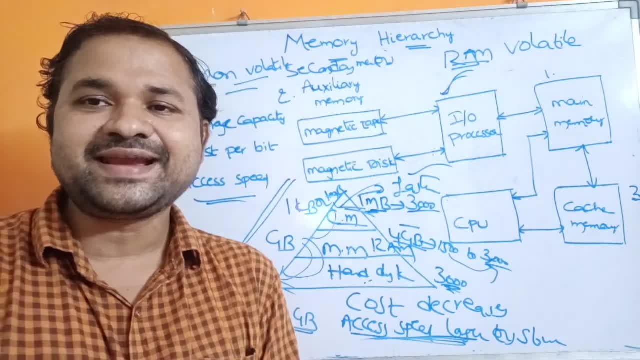 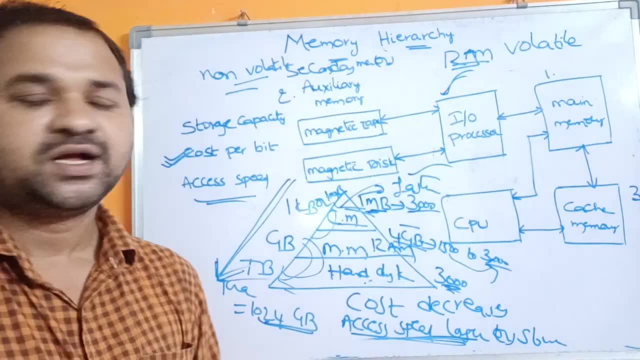 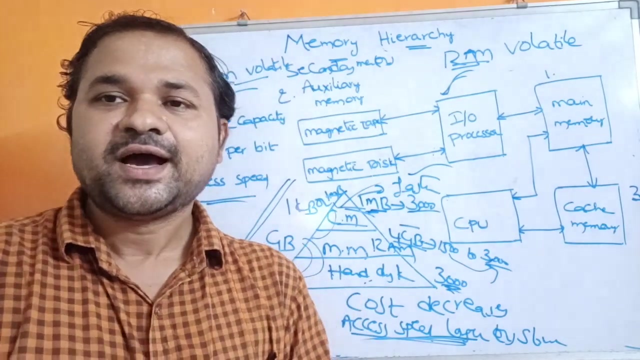 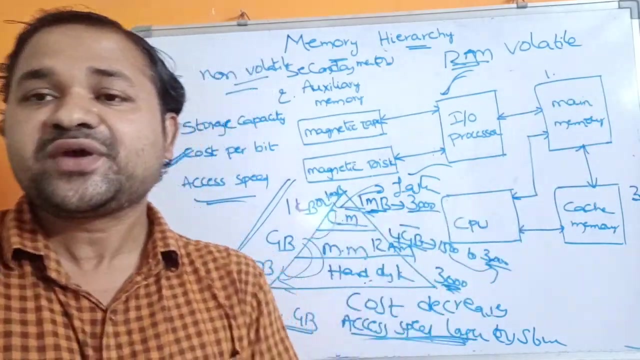 multi programming means multiple programs can resides in the main memory simultaneously. so if one program is waiting for i o operation, then cpu allocate the task to i o processor and cpu starts executing some other program. here the cpu access time is very, very faster, whereas the main memory access time is very, very slower. so in order to compensate the difference,